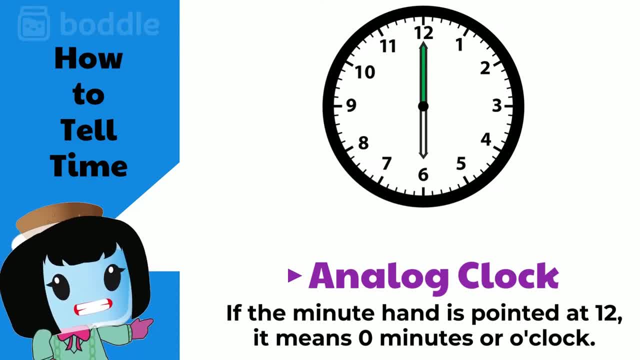 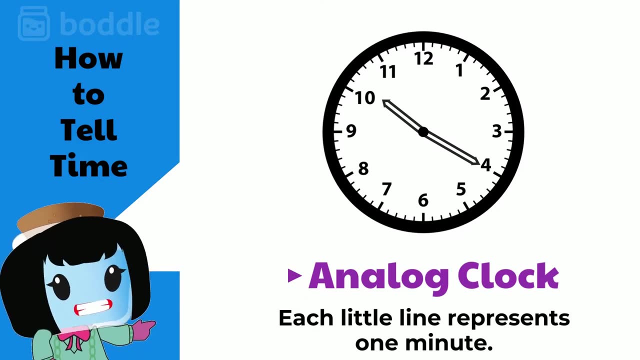 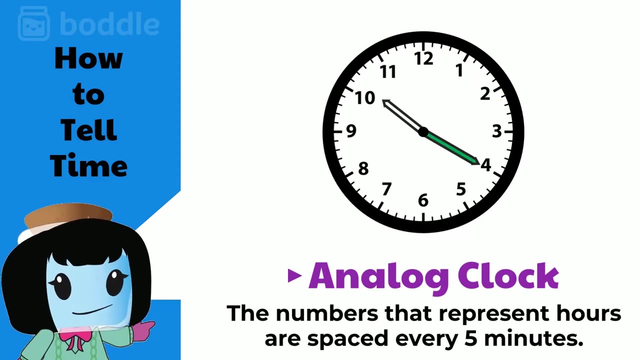 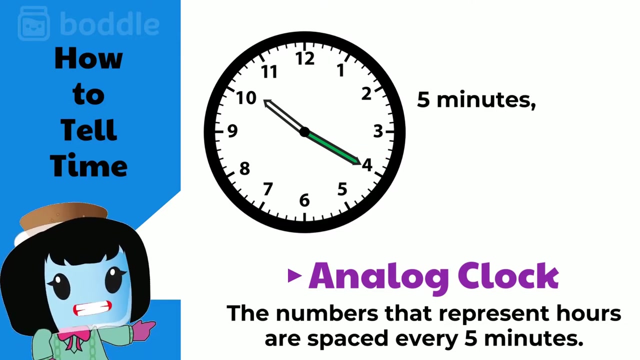 minute hand is pointed at 12, it means zero minutes or o'clock. after that each little line represents one minute. the numbers that represent hours are spaced every five minutes. so if the minute hand is pointing at the four, it is the same as five minutes four times or 20 minutes. 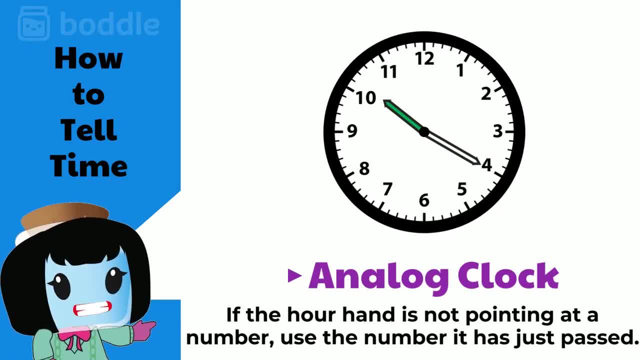 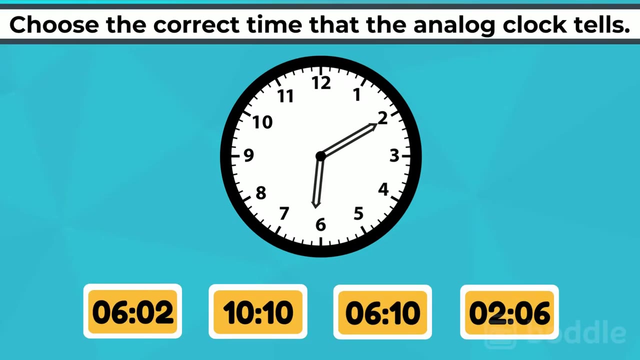 sometimes the hour hand will not point exactly at a number. in this case, use the number that the hour hand has just passed. let's test our clock telling skills by choosing the correct time that the analog clock tells. The hour hand is pointed between 6 and 7,, which means it just passed the 6,, while the minute hand 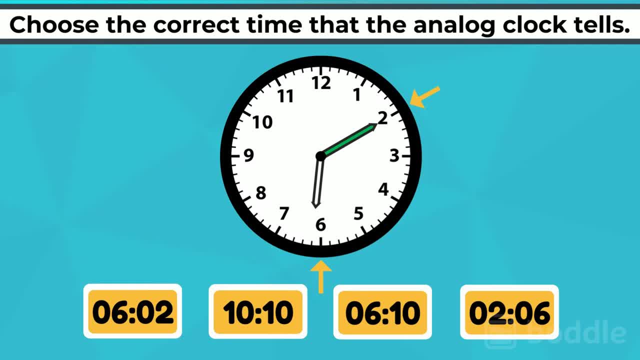 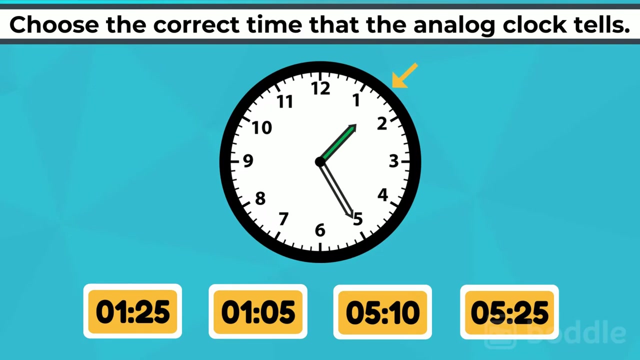 is pointed at the 2.. Remember, with the minute hand each hour number represents five minutes. So if it's pointing at the 2, that means it's 10 minutes. So the clock says that it is 6.10.. On this one, the hour hand is pointed between 1 and 2,. 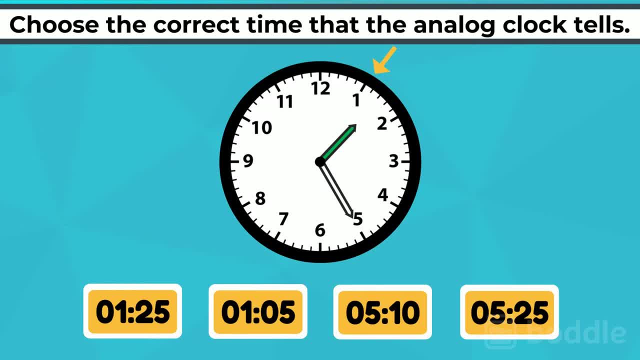 meaning it has just passed 1.. The minute hand is pointed between 1 and 2,, meaning it has just passed 1.. The minute hand is pointed at the 5,, which means 25 minutes, So the time is 125.. On this clock both. 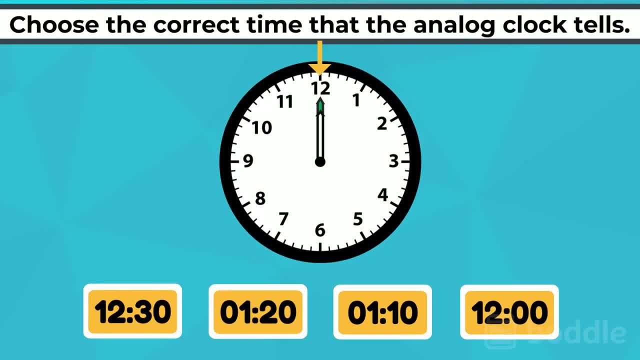 the hour and the minute hands are pointed at 12.. That one's easy. The time is 12 o'clock. On this last one, the hour hand is pointed between the 4 and the 5, meaning it is just past 4, while the minute hand is pointed exactly at the 6,. 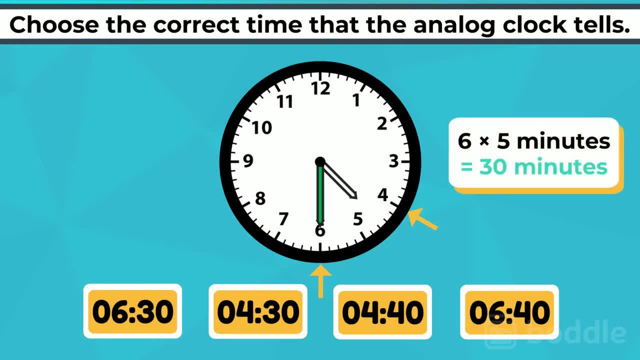 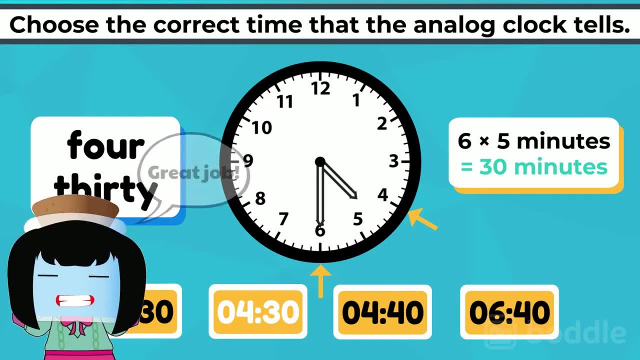 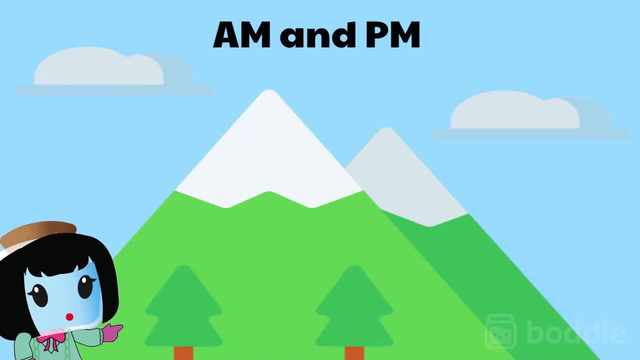 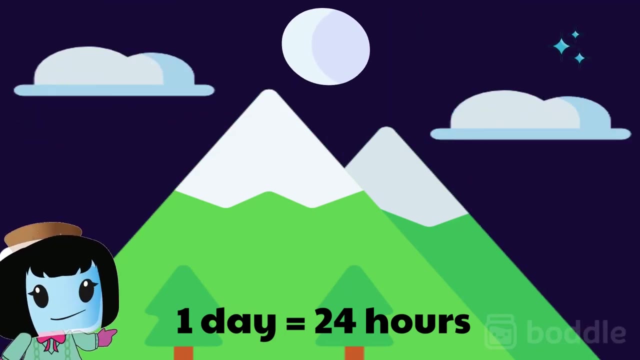 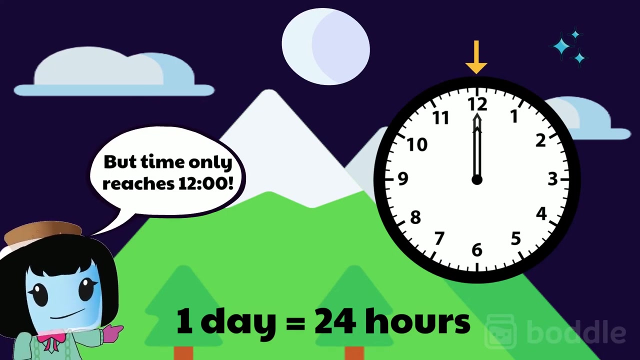 which represents 30 minutes. So the time is 4.30.. Great job reading those clocks. So let's talk about whether it's am or pm. Remember a whole day is 24 hours, But did you notice that our time only reaches 12 o'clock? After 12, it goes back. 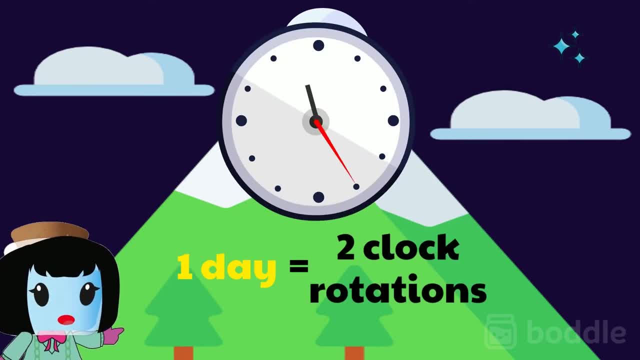 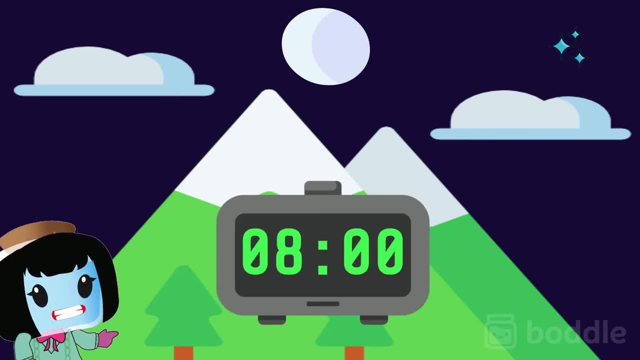 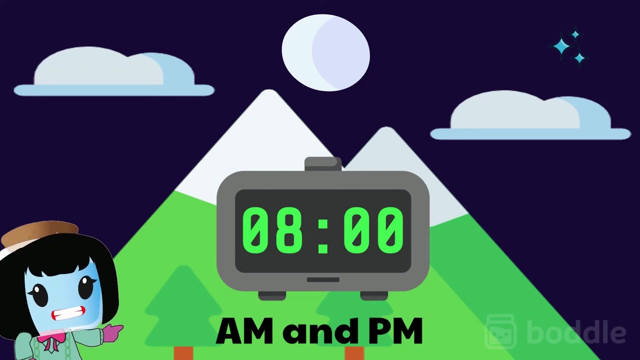 to 1.. It means that a whole day does two rotations on our clock. So if we say 8 o'clock, it could be in the morning or in the evening. So how do we know which it is? This is where am and pm help us out. Am is used for any time after midnight. 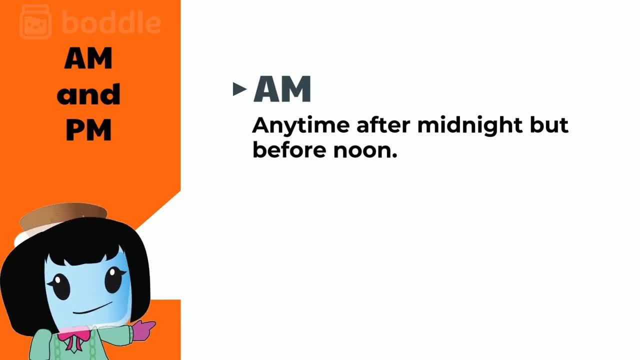 but before noon. Well, pm is used for any time after noon, but before midnight It's also used for some other time after noon. Just keep that in mind. Let's look at some examples, just to make sure we understand. 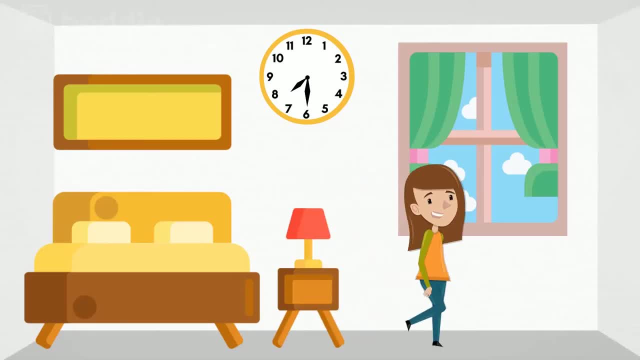 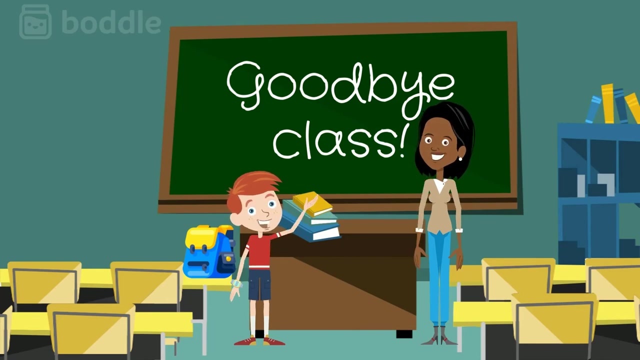 Tina wakes up in the morning and sees her clock. What time is it now? Well, her clock says 7.30, and since it is morning, the time would be 7.30 am. Darrell finishes school in the afternoon. He checks the time to see if he can still. 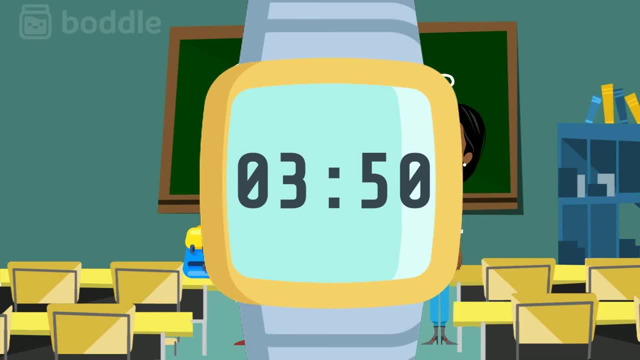 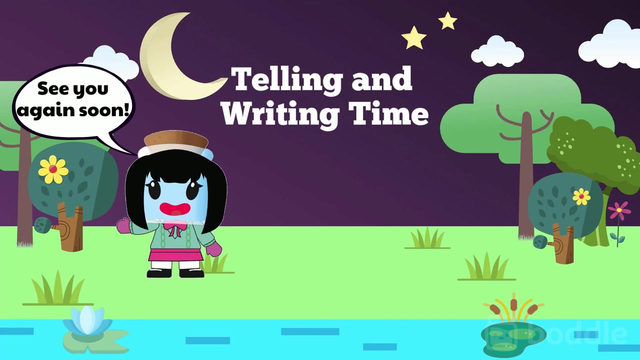 watch his favorite TV show. I've changed it to am, And pm is used for any time after noon. favorite show. What time is it? The clock says 3.50.. And since it's in the afternoon, the time is 3.50 pm. Great job working on telling and writing time. See you again soon. 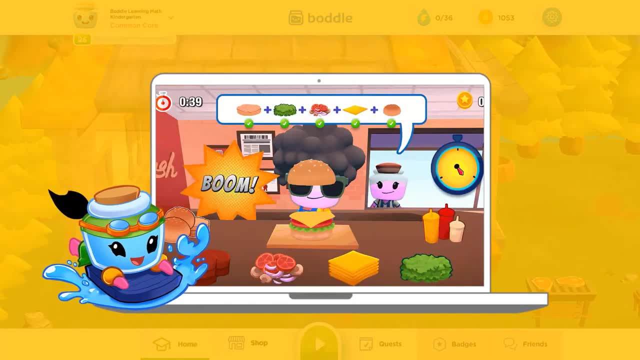 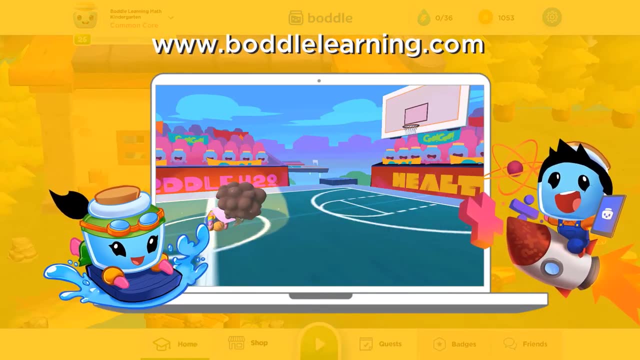 Are you looking for more fun ways to learn math? Check out Bottle Learning and access thousands of math skills all through a fun 3D game. Just visit BottleLearningcom and sign up today.